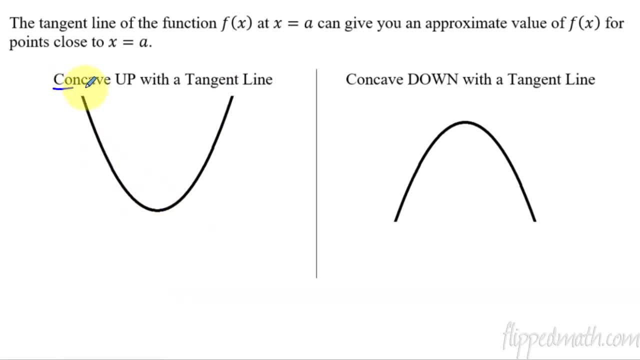 down. For now, in this lesson, I'm just going to tell you- I'm going to give you these words- that a function is concave up or that a function is concave down. so you don't have to worry about figuring that part out. It's part of the problem. What I want you to do is pick any point along. 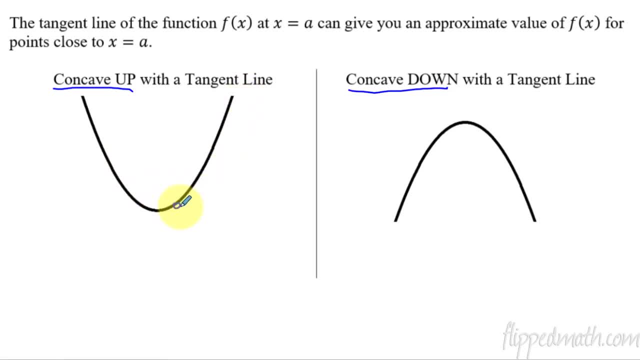 here, probably down here somewhere on the curve, just pick a point. I'm going to choose right there and I'm going to put a dot, and then I want to draw a tangent line on that dot. So try and draw a straight line. see, okay, that was awful, let's try again. okay, that's better. So I have. 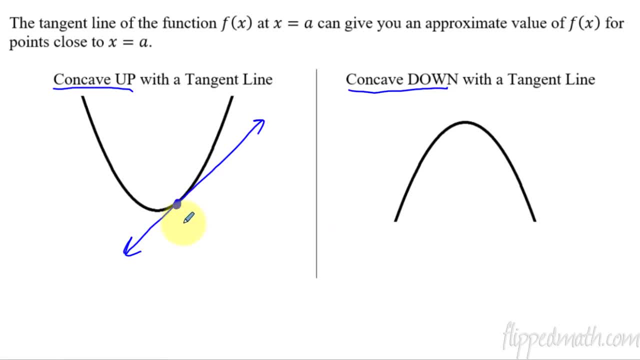 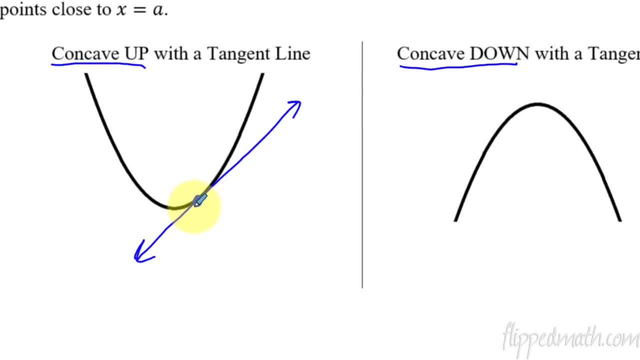 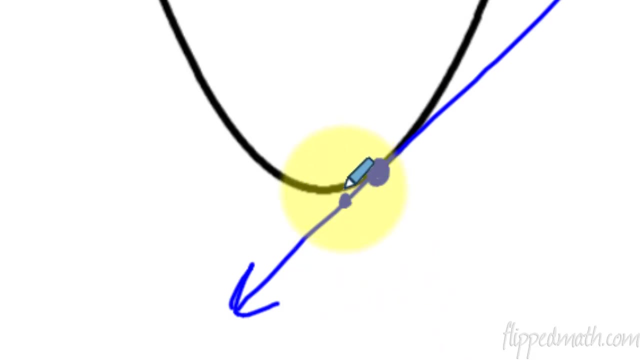 a tangent line that's going off here, and if I were to be able to take a point that's really close to this- this is kind of like my x equals a that I'm talking about up here- If I took a point that's really close, like let's say right there that little dot would be an approximation of the function. 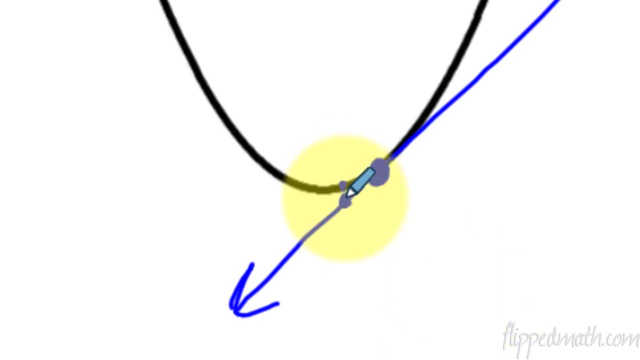 that's right above it at that same x value. See how they're close to each other. they're not the same but they're close. So again, if I took a point right here, that would be an approximation of the function right there. and the further away I get from the function, the further off my approximation would be. 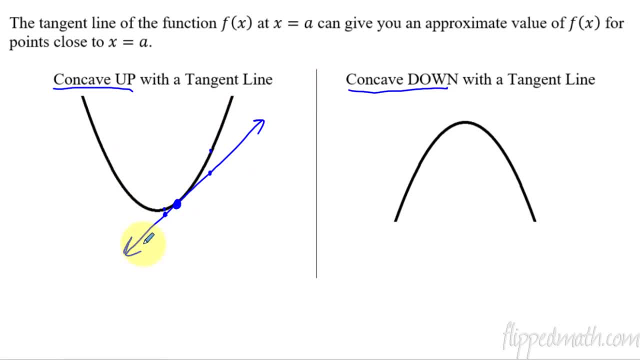 So that's what we're going to be doing today. Now, the reason this concave up is important is because it tells you whether or not it is an overestimate or an underestimate. So if you look at this line, everywhere on this line, it's underneath the function. What that means is that 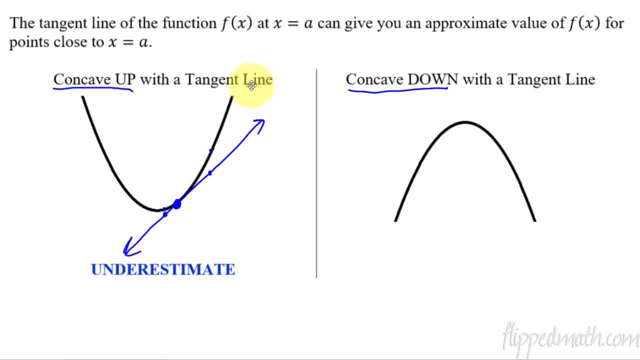 if the function is concave up. a tangent line gives you an underestimate of the function. Okay, let's go to the next one. Concave down, Do exactly the same thing. Just want you to draw a point anywhere along there. Just pick a point, draw a line and okay, there we go. that works, and then we're doing the same thing. 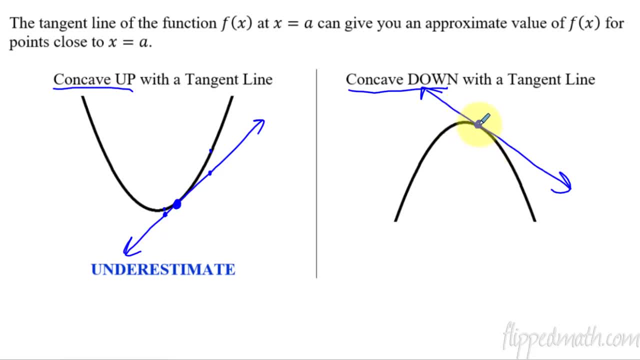 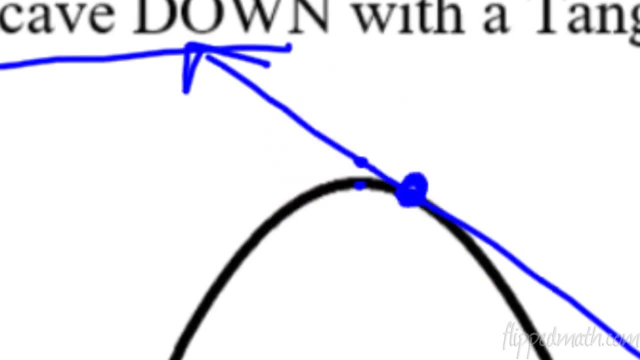 we did before, and that is, if you just choose any point that's right around this, x equals a dot. if we choose a point like right here, you can see that would be an approximation of that point right there. That's what we're doing And, in particular, is it an overestimate? 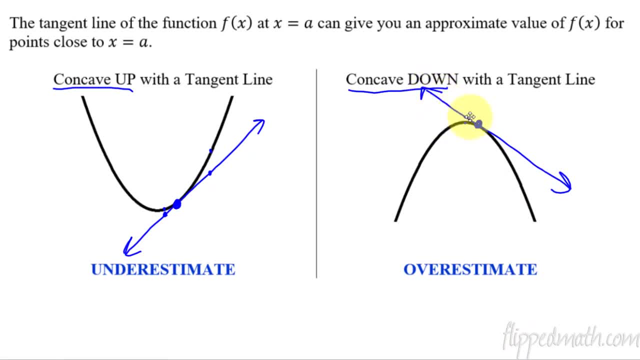 an underestimate. it is an overestimate. every single point on this line is going to be above the function. well, except for the tangent line- the tangent point, I should say, but all the rest of these that we were using for an approximation would be above the function, and the further away we get from that point, the 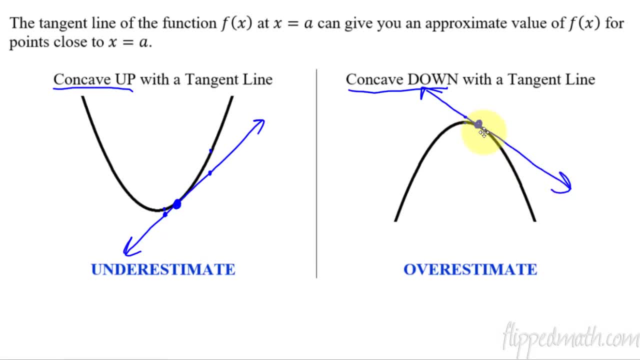 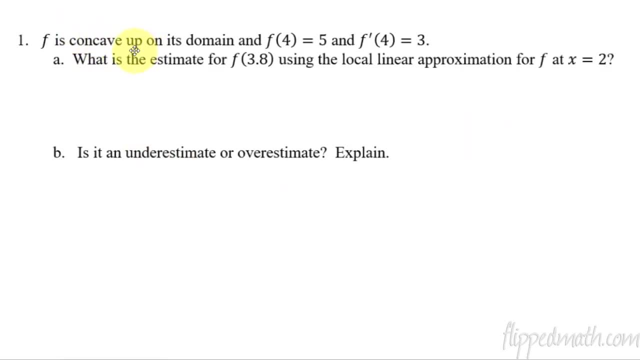 worse of an approximation it would be so you want to stay close to that little dot right there. let's put it into practice. here we go. number one F is concave up. see, you don't even have to figure out if it's concave up, I'm just. 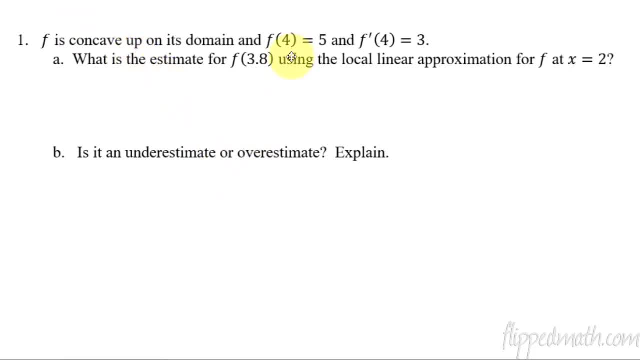 gonna tell you that. so it's concave up on its domain. and f of 4 is equal to 5, f prime of 4 equals 3. so that just tells us. we have our coordinate point 4, 5, and we have the derivative, or in other words the slope of the tangent line at x equals. 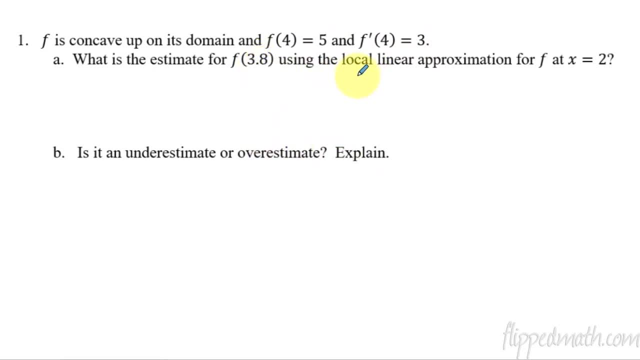 4. so what is an estimate for 3.8? using this thing called local linear approximation, that's, using the tangent line to give us an approximation. local linear means, if you know, if you think about you zoomed way in on a function, it looks like a line right that might be curved, but if you zoom way in it's. 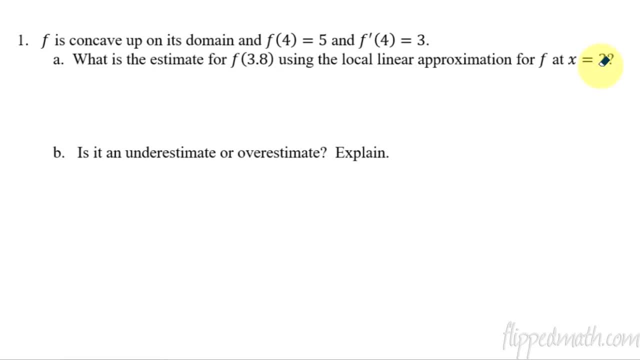 actually gonna look like a line. oops, you're notes will be right. I'm going to fix that. sorry, I should have said at x equals 4. I'll fix that and your notes gonna be correct, okay. so what is the estimate for 3.8? well, first we have to come up with a 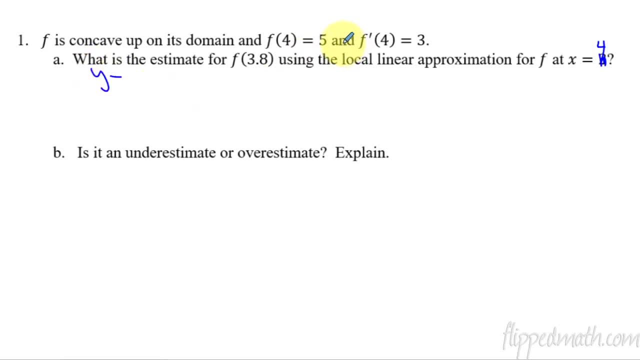 tangent line. so let's do that: first y minus what's my. my y value 5 equals, and then my slope is 3, because that's the derivative 3 times X minus 4. okay, we've been doing that for a while now. there's our tangent line. you could solve for Y. 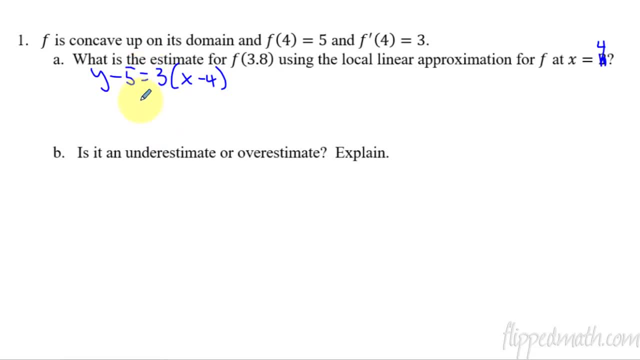 if you want- it's not necessary to- you could use either this or you know, or we could. uh, y equals 3x. distribute that negative 12, add the 5. negative 12 plus 5 is negative 7. so you could use either one of these. it's actually probably easier. 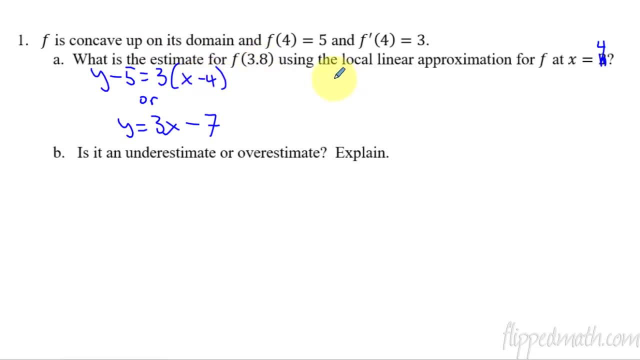 to use this first one, and i'll show you why- because now we're going to use 3.8 and plug that in to the line and see where is this line at. x equals 3.8. so i'm going to go 3.8 minus 4 and 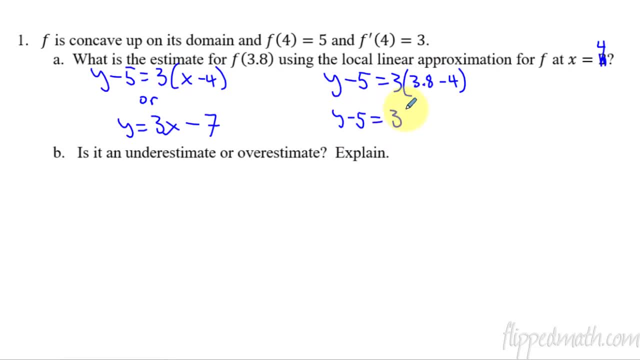 then i have y minus 5 equals 3 times, and this is just negative 0.2. so see, this is a little easier to do without the need of a calculator. you can use a calculator on this and then that's just going to be: y equals 4.4, and i'm cheating because in the background i'm using a calculator. okay, so 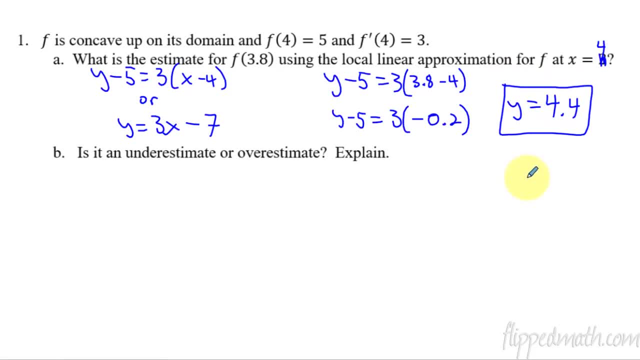 4.4. this is an estimate of the actual function. we don't even know what the function is. we just had some information about it. so now let's go to: is it an underestimate? over over estimate and explain concave up, it's concave up. 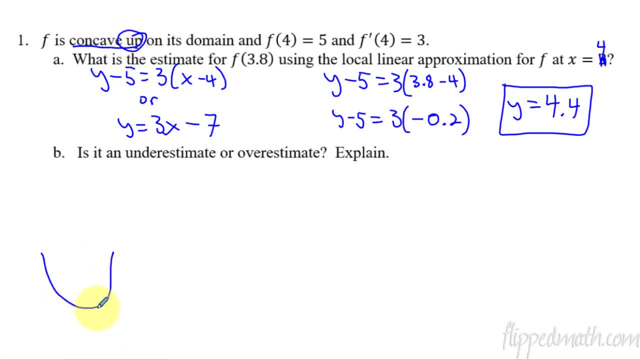 so what do we have going on here? we have something like this. we have some tangent line taken off like that and we are using: oh, that was awful. and then we have: we checked: this is at: x equals 4. we checked at 3.8. we got an answer of a y value of 4.4, but this whole line is underneath it. so this: 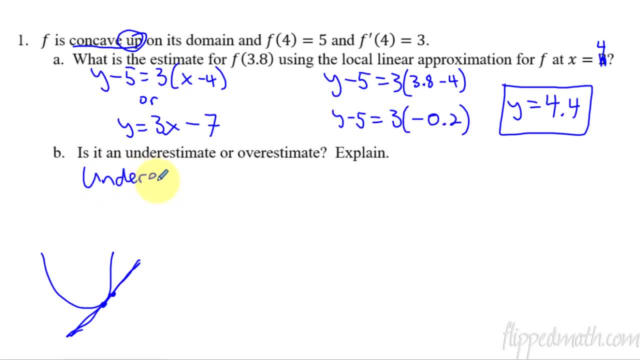 is an underestimate. so this is what you say: underestimate, if i can write here, because f of x is concave up. that's why it's an underestimate, because f of x is concave up, and that's all you have to say. that's how we know that that value is an underestimate. next problem, number two: so we've 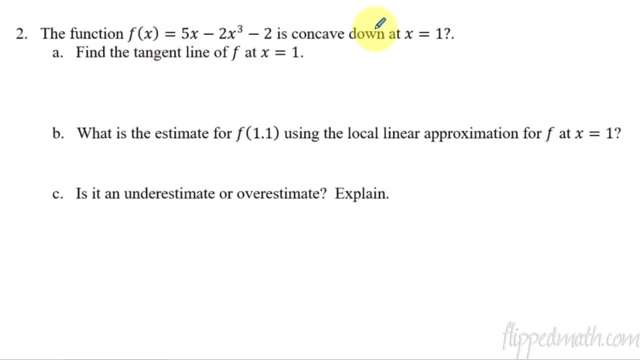 got now the actual function and we know that it's concave down at x equals 1, so let's find the tangent line. so remember, we need uh, we need x1, we need y1 and we need slope, which the slope is the derivative. so we already have the x1, we know that's a 1, we need the x1 and we need the slope. 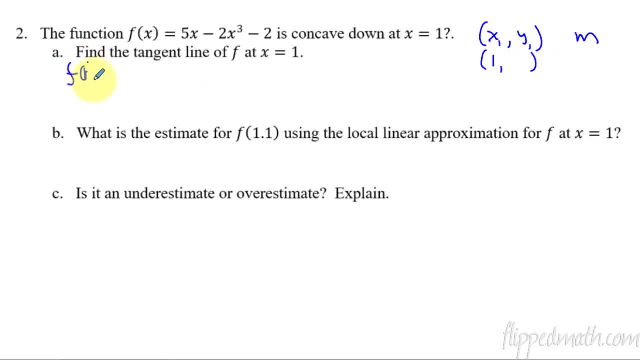 the y value. so let's figure that out first. f of the number 1 is going to equal 5 times 1 minus 2, times 1 minus 2, 5 minus 4- hey, it's also a 1, okay, so the y value is a 1 as well. now let's do the. 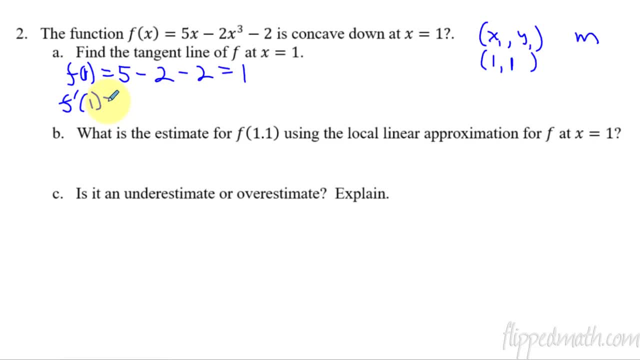 derivative, the derivative with a 1 plugged in. i think we can do this all in one step. the derivative of 5x is just 5 minus 2x cubed is 6x squared, and i'm plugging in a 1, and then the derivative of: 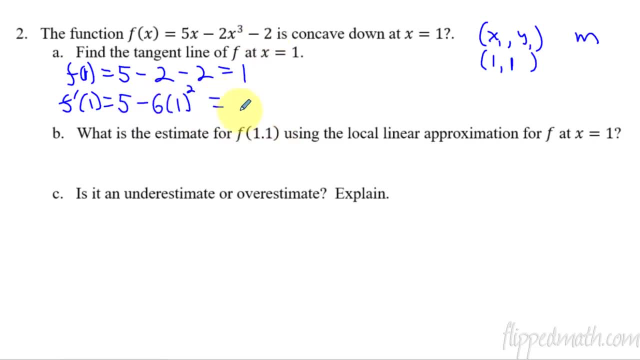 minus 2 is nothing, it's 0.. so now i have 5 minus 6. it equals negative 1.. all right, so my slope is negative 1, and so now i can do the line y minus 1 equals negative 1 and then times x minus 1.. okay. 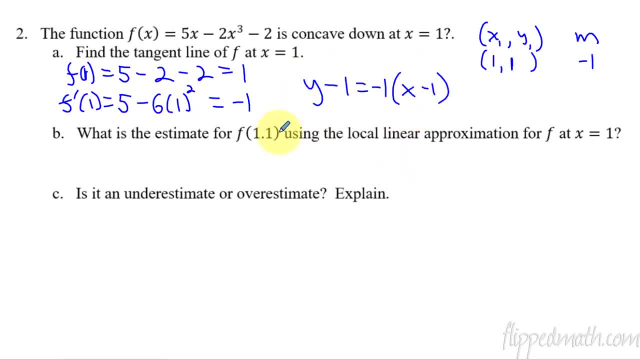 there's my line again. i still think it's easier to use this form when you have to plug in a number, uh, like a 1.1. you'll see here on this next one. so what's the estimate? we plug in a 1.1 y minus 1. 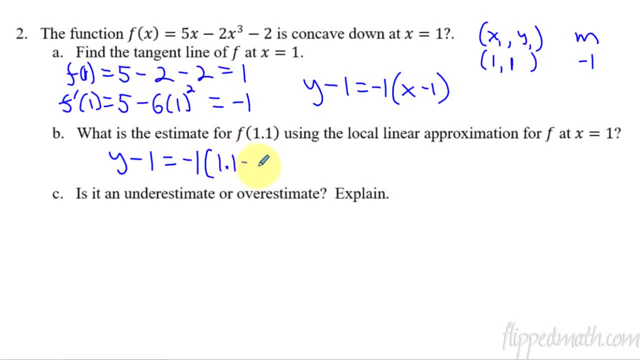 equals negative 1 times 1.1 minus 1.. so then let's go over here. what's this become? y minus 1 equals 1.1 minus 1 is 0.1 times negative 1, so negative 0.1. add 1 to both sides and we get y equals. 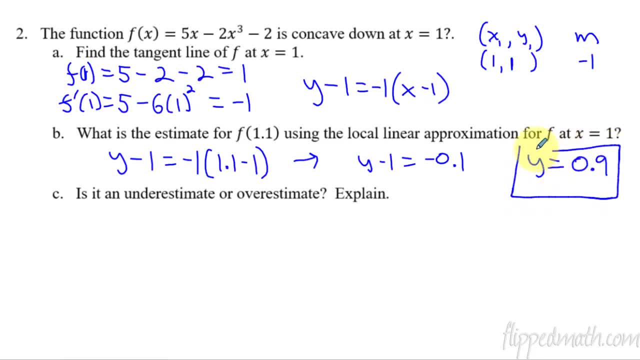 0.9. that is my estimate that the tangent line gives me for what the actual function is. now we could plug in a 1.1 and see exactly what it was if we wanted. but that's not the point of this. we're trying to see how the function works, so let's plug in a 1.1 and see exactly what it was. 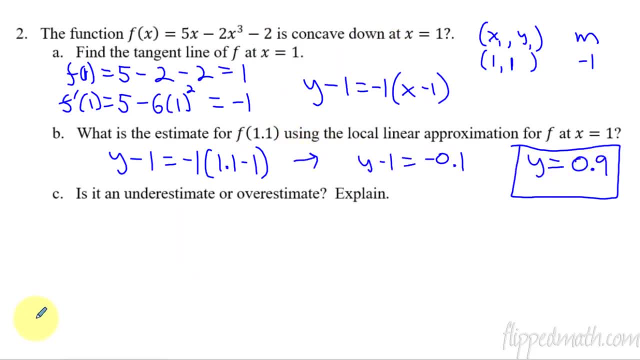 how the tangent line can help us get an approximation. and then i know it's concave down. so now again, if it's concave down and i have any tangent line i want on this thing, if it's a tangent line, then we know that this is an overestimate. the line is above the function. 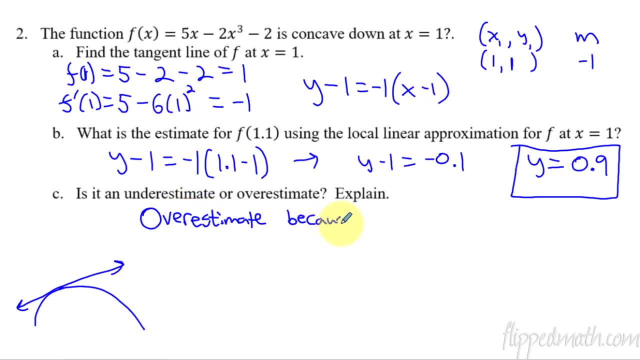 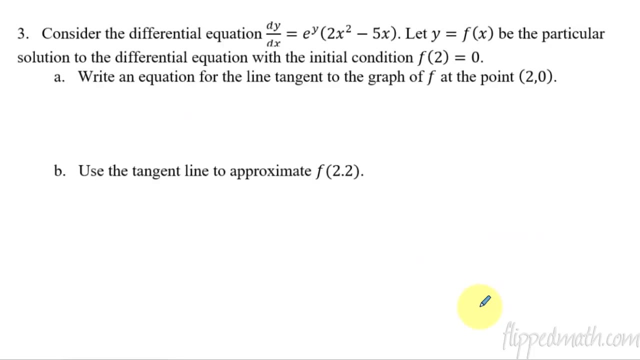 so over estimate, because f of x is concave down, and that's your justification. you're explaining why this is an overestimate: because you know the concavity, so the tangent line had to be above. that's what that means. last problem, here we go, this last one here. now i'm giving you a differential. 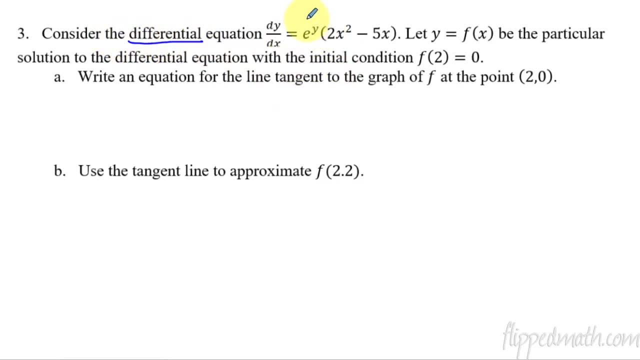 equation. a differential equation is just like the derivative of when you do implicit differentiation. remember when you we back to when we did implicit differentiation and you solve for d, y, d, x. okay, that's a differential equation. now, what's this weird stuff here? let y equals f of x be the. 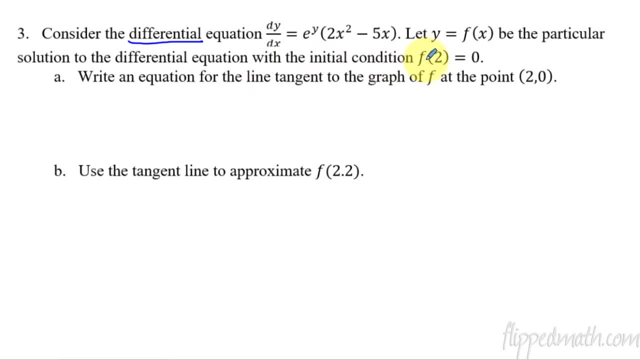 particular solution to the differential equation, with the initial condition f of 2 equals 0.. okay, that looks really confusing. this is a little bit confusing, but it's a little bit confusing, so let's see what this means. if you have the y equals f of x is the particular solution of what this used to. 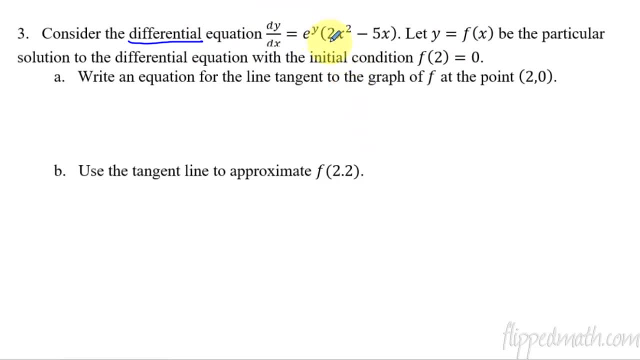 be before we took the derivative. so if we like, did the anti-derivative- which is actually a real thing- we'll do that later this year. if you went backwards, you'd end up with this: okay, we don't care what it is, it doesn't matter. all we're telling you is that it exists and you know that this point happens. so 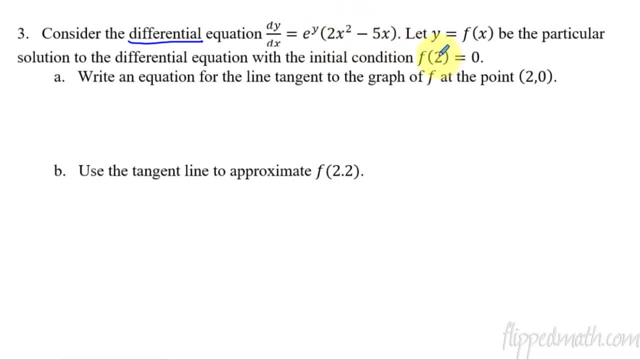 if you were to take the anti-derivative and figure out what the actual real function used to be, and you plug in 2 into the x, x, then these: y is a zero, x is two, y is zero. that's all. this is okay, so let's do this write.